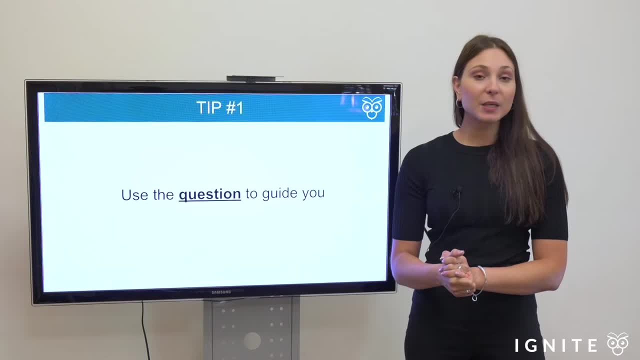 When you go into your comprehension papers or whenever you're looking at unseen texts generally, it's absolutely crucial that you look at the questions based on that text first. Often the text will actually give you the question. sorry, will give you an insight to what that. 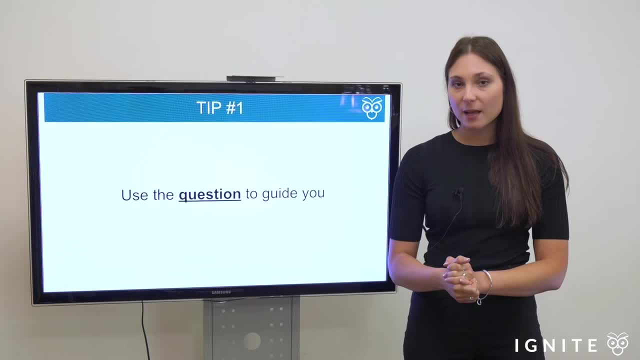 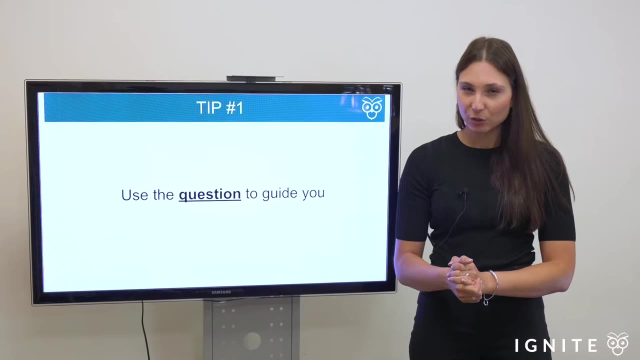 text is about and what you're looking for in that text. The question will also give you the mark allocations for that particular text. in answering that question, The mark allocation is important because it's an insight to how much evidence you need from that text when you're responding to it. 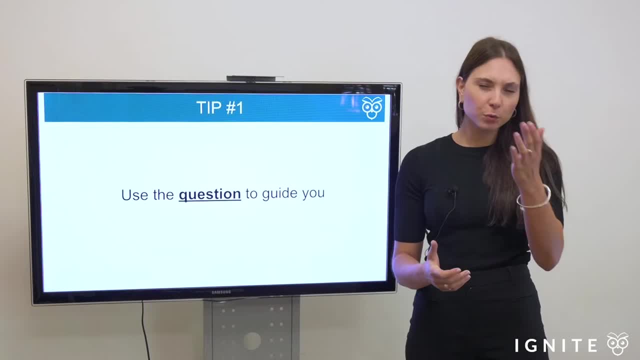 So if it's a four mark question, you're looking for about three quotes. General rule of thumb, by the way, is marks minus one is how much evidence you should be using, So use the question to guide you. The question is going. 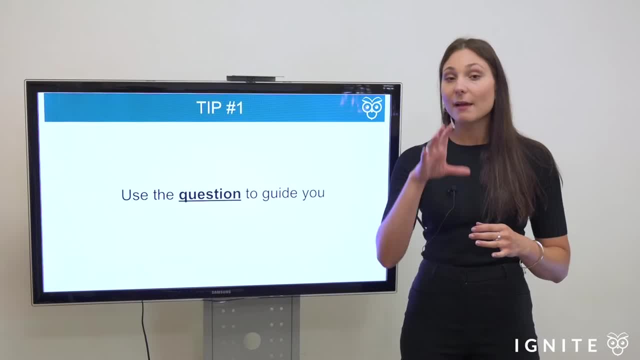 to tell you what kinds of ideas we're looking for in that text, and through knowing the ideas, you're already getting a bit of a picture of what that text is about. If it's quite a long text, you're only answering a two marker. that also tells you that we don't need to dwell too much. 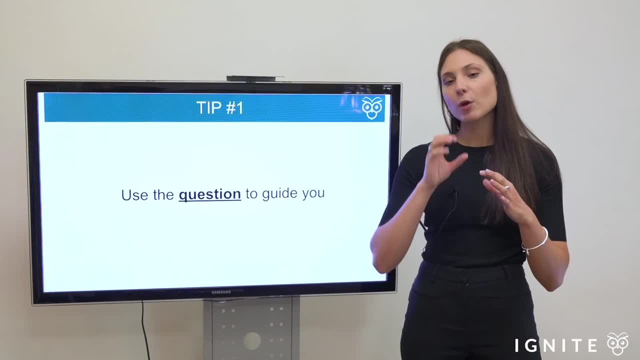 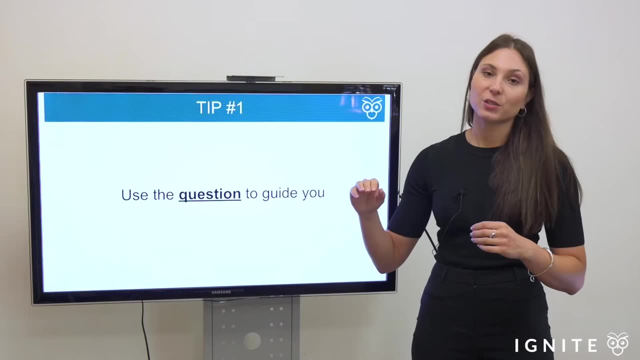 on looking at this particular text. We can afford to skim through, pick out the quotes that are necessary and be efficient with your time. So, tip number one: use the question to guide you. Use it to help you work out what the key. 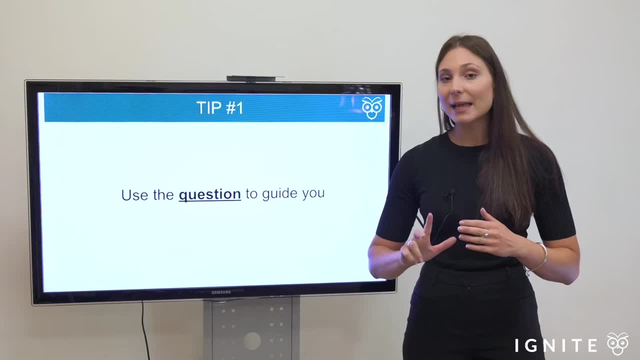 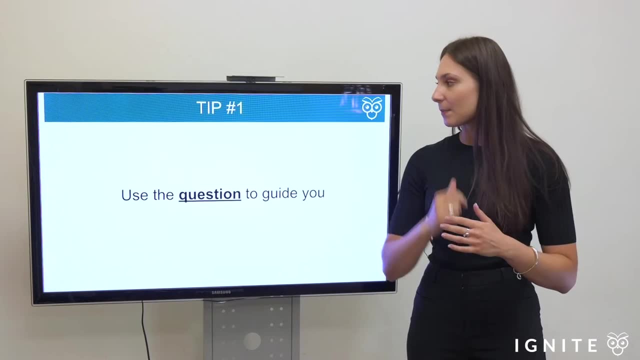 themes are in the text, know how many quotes to use and to give you a bit of a feel of the kinds of ideas that you'll need to be extracting from the text in order to answer your question. So that's tip number one. Tip number two: look actively for the number of quotes necessary. 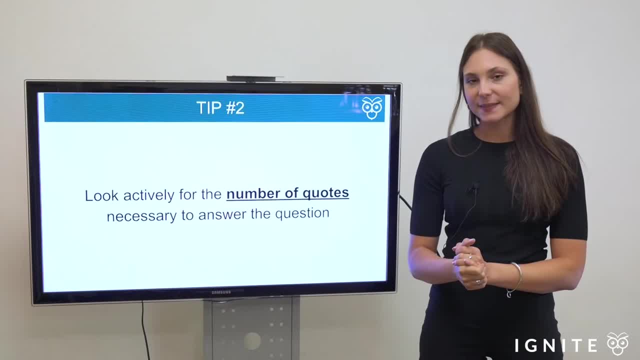 to answer the question. So this is a bit of a segue from my previous slide. I think it's important and I do come to this a lot when I'm answering questions. but I think it's important- and I do come to this a lot when I'm answering questions, but I think it's important and I do come. 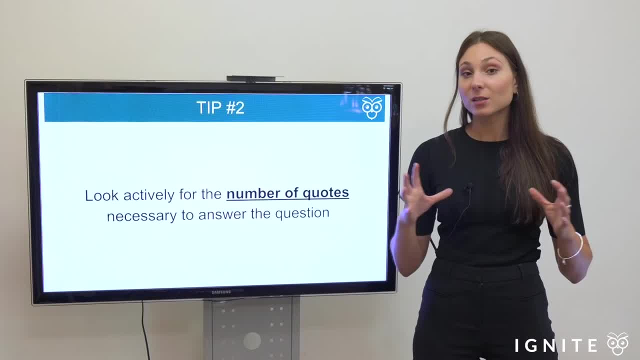 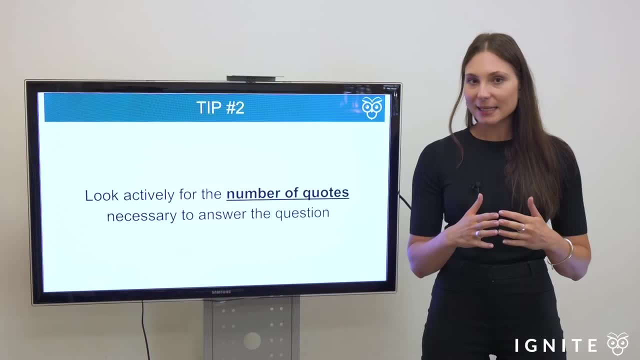 to this point later on to consider how. you don't need to look at the text and feel like you're understanding every single line, every nuance, every technique. Responding to unseen text is a very strategic process. You're looking through and you're wanting to just quickly extract. 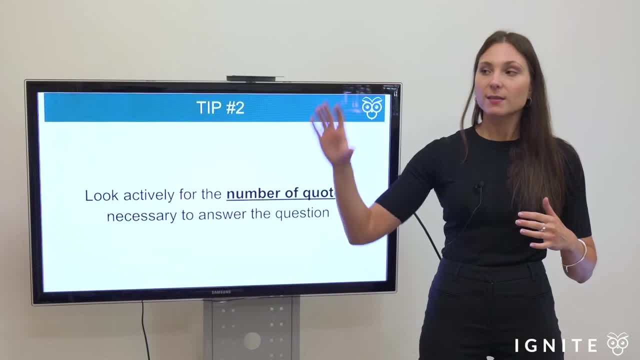 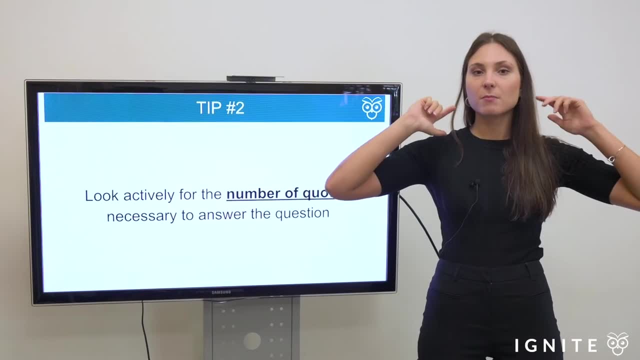 the quotes that are necessary for you to answer the given question. So, looking at the mark allocation, looking at the question itself, from those two things alone you're thinking, okay, which quotes are going to be most relevant to me answering the given question. And you have to very quickly navigate through the text in that. 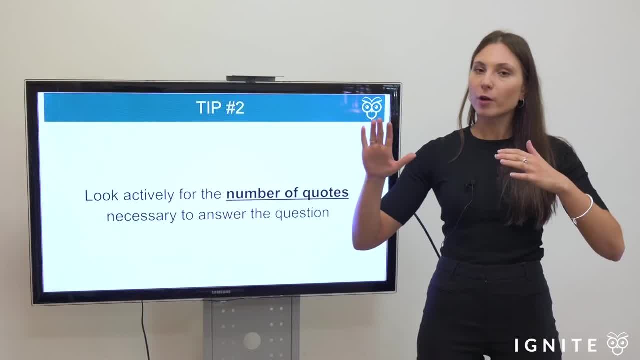 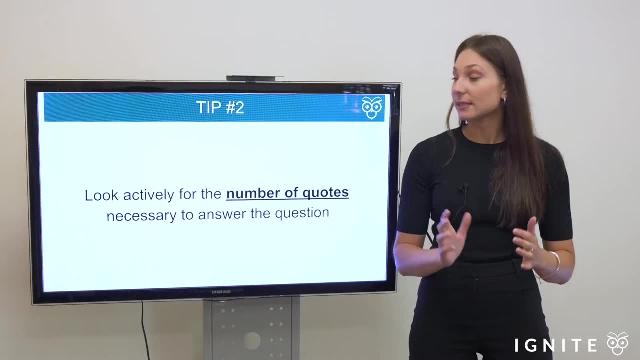 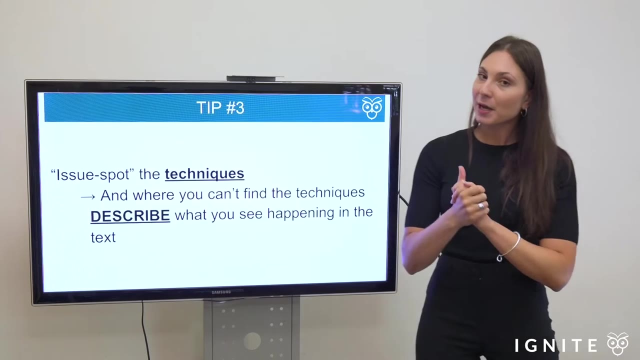 particular way. So actively look for the quotes. Don't feel burdened to work out exactly what the meaning is behind the text. Just work your way through and very quickly take out what is necessary. Okay, tip number three: issue spot the techniques. And where you can't find techniques, describe. 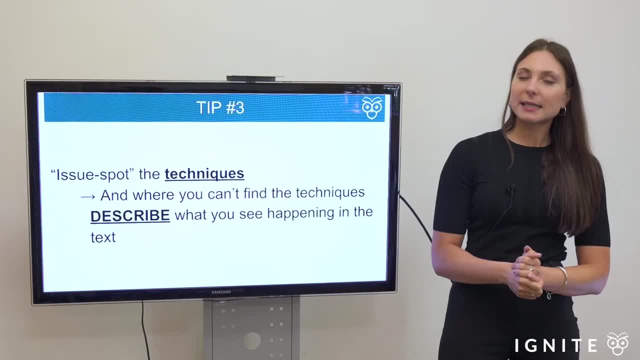 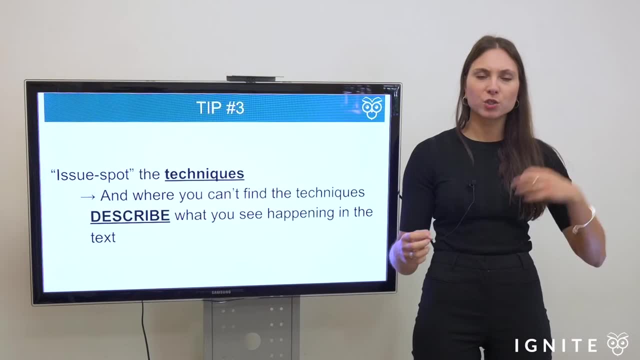 what's happening. I often find that when students are looking at unseen text, they get really panicked that they can't find the typical techniques that they would usually call upon. The metaphors aren't jumping out at you, you don't see personification, you can't spot the sensory imagery, and that's. 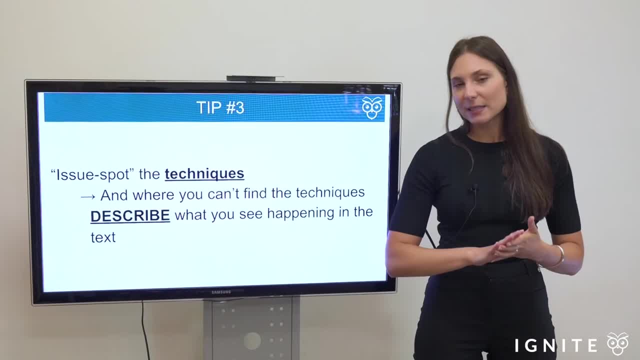 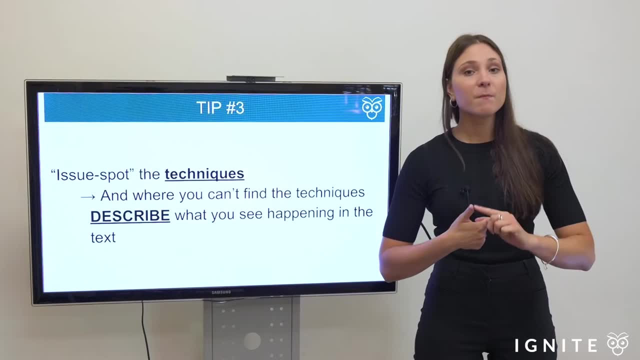 okay In that case. by the way, come back to a couple of basic techniques. I have a bit of an acronym for written text that I think is really useful. The acronym is MEST M-E-S-T- M for modality, E for emotive language, S for syntax and T for tone, And you'll notice, with those four. 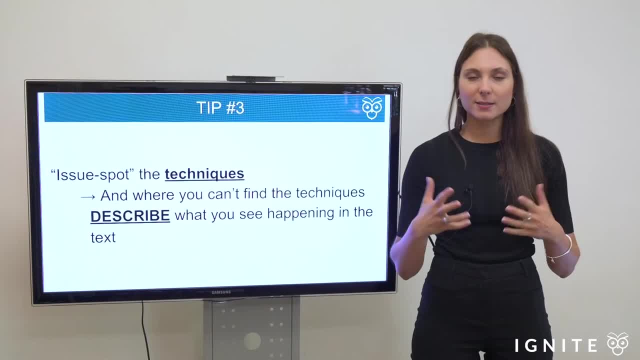 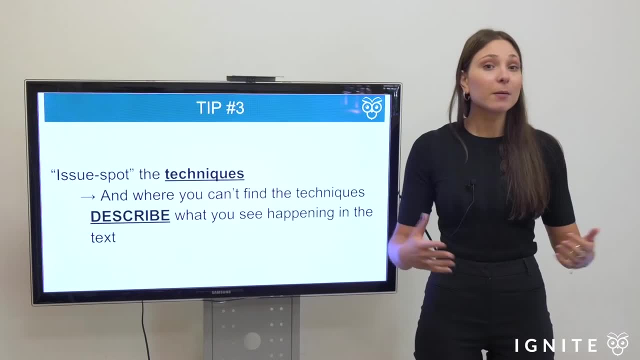 techniques I've just listed there. they're kind of like go-to techniques. There's always going to be a tone that's conveyed in what's being written, there's always a certain level of modality, there's always potentially an emotion that's being conveyed and syntax is relevant to. 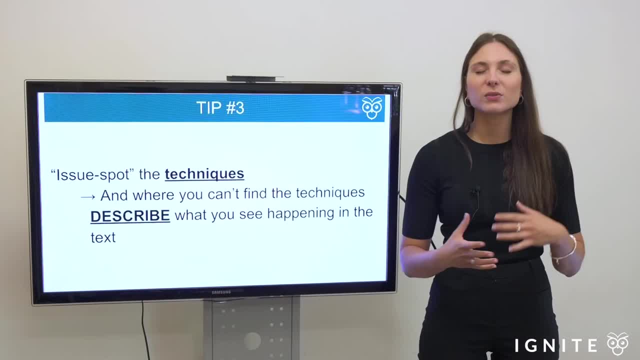 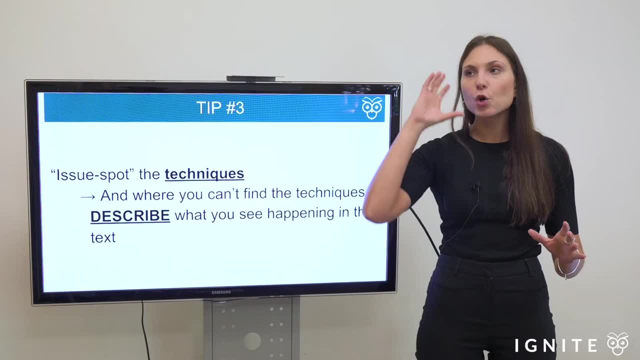 every sentence, because you're considering the sentence construction, the uses of pause, the word order and so on. So come back to those techniques. But nevertheless, even when you can't find the techniques in the text, if you're noticing something about the way the text is being written, 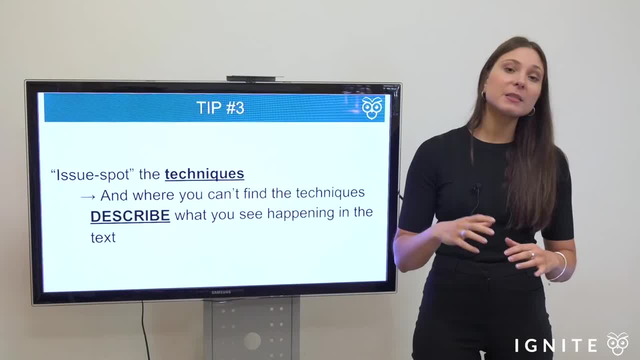 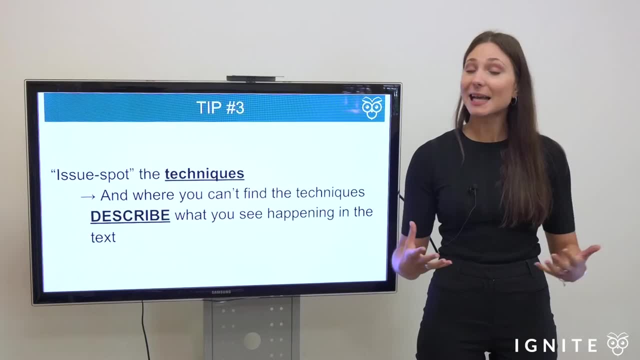 describe how you see the language unfolding, If a particular voice is being used, or if the text is fast-paced or if the text is a little bit slow. or if the text is a little bit slow, or if the text is, if it seems kind of fragmented or even jumbled, if the sophisticated words you usually use to 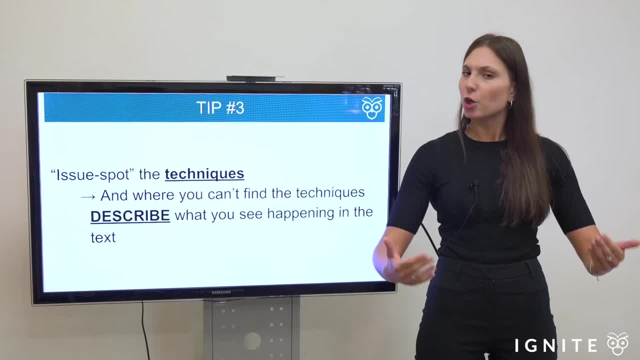 describe language aren't coming to you. strip it back, don't put so much pressure on yourself and just describe what is happening within the text, And when you do that, it enhances your analysis ability and you don't feel so pressured to categorize through using techniques what's? 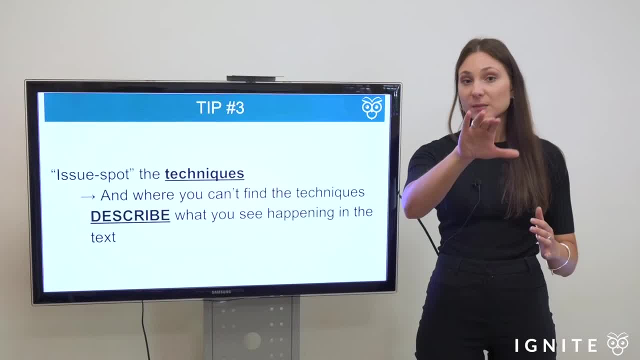 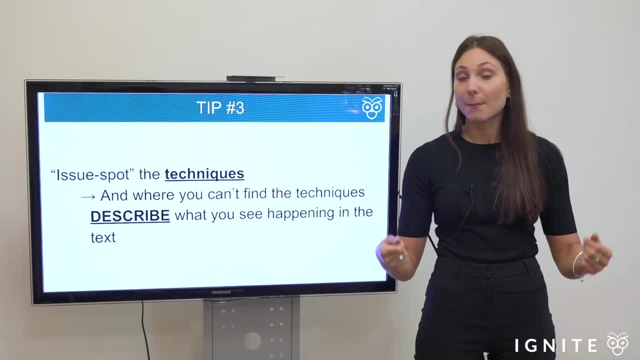 happening in the text. So, of course, focus on issue spotting, try and find those techniques, but if you can't, at least describe how the language is working in the text, and that will give you some marks because you're still considering the construction of the text. 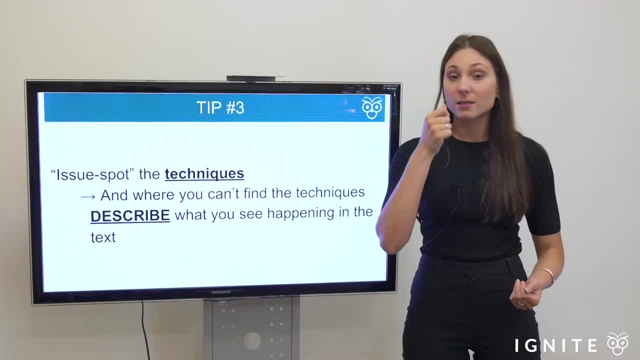 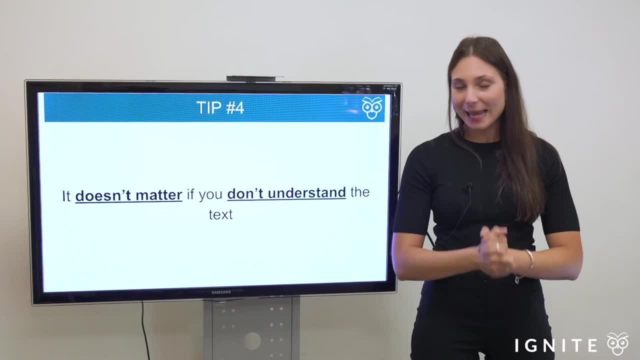 and just because you're not labeling a technique doesn't mean you're not analyzing. So that's an important bit of advice as well. All right, tip number four: Yes, if you don't understand the text, it doesn't really matter. Remember, you're not writing a. 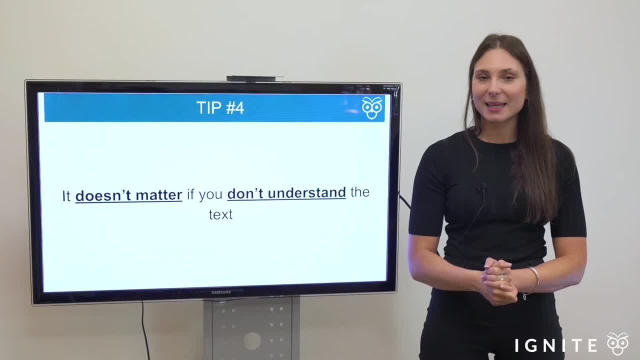 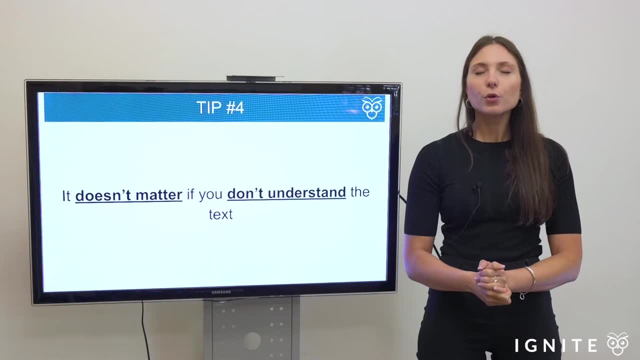 full-on dissertation or huge essay on this unseen text. The approach here is for you to answer a question that is most likely a maximum of seven marks. Okay, so all you're really looking for are extracts that you can link to given themes that have been framed in the question. 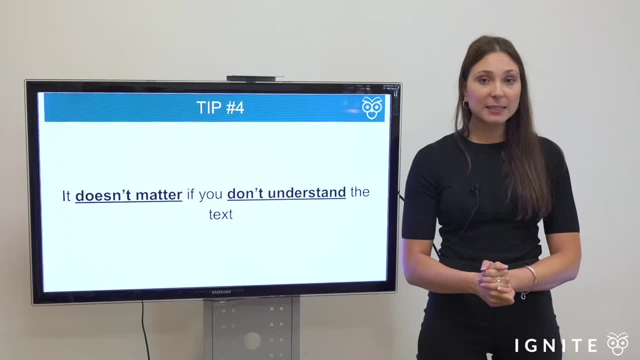 It's really the process of extracting evidence, identifying a technique or describing what you see in that particular quote and linking it back to the question. So when you're looking at these texts, don't look at them with the critical lens that you need to unpack very deeply what the 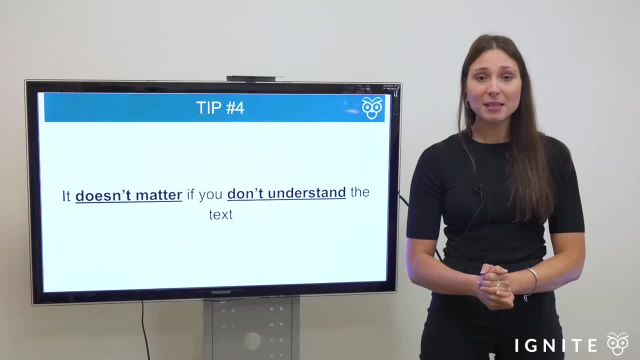 hidden meaning is in there. It might be the case that there is no hidden meaning in the text. You might be given an extract from a larger piece, which means it's impossible for you to work out the overarching meaning that can be found in the text. So if you're looking at the text, you're 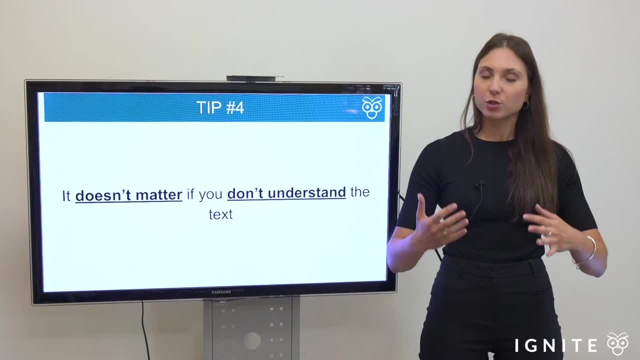 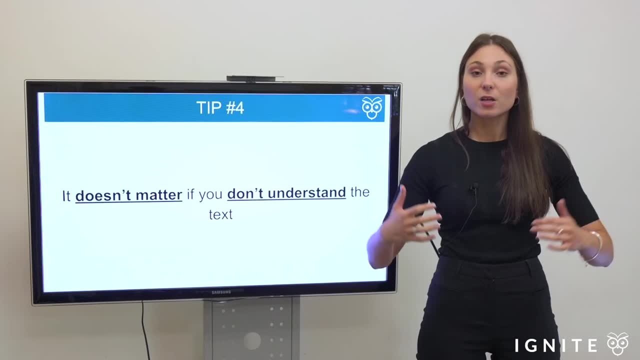 looking at what the composer is trying to convey. So shift your focus. You're being strategic, You're picking out the best quotes, linking them to the question and not getting lost or burdened by the desire to know fully what the text is trying to convey. Liberate yourself issue spot. find the 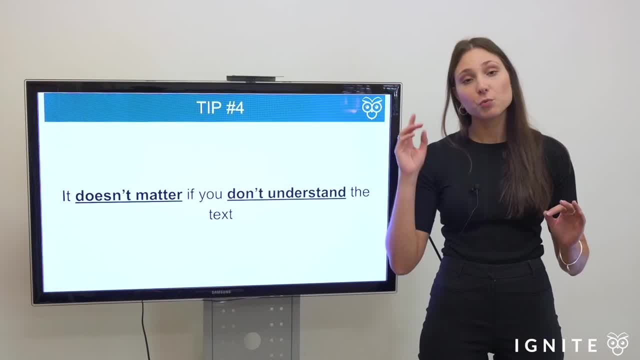 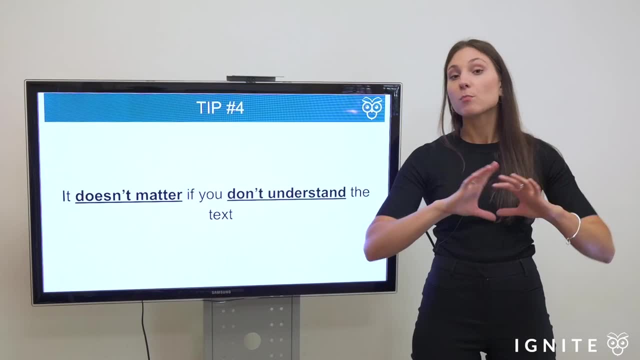 quotes and just sufficiently answer the question and move on. You will not have time to waste if you are looking at unseen questions and texts in the comprehension exam, But this advice, of course, is applicable more broadly to anyone analysing the unseen text. 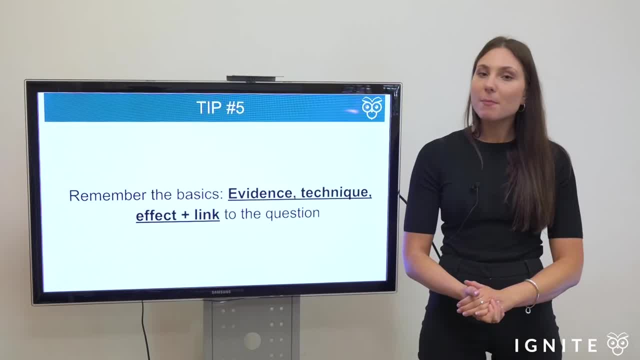 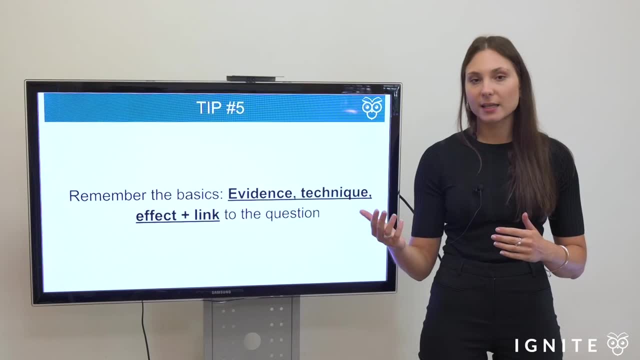 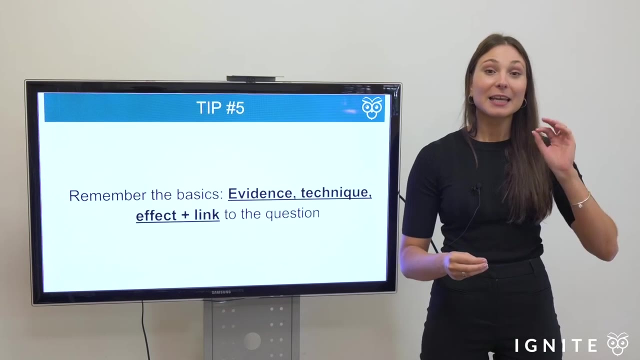 And our final tip is: remember your basics. At the end of the day, the marker is looking for evidence, technique or form effect link to question. Tattoo that sequence onto your mind. When I'm teaching younger students, it's quite common to see them forgetting to actually give me the quote. 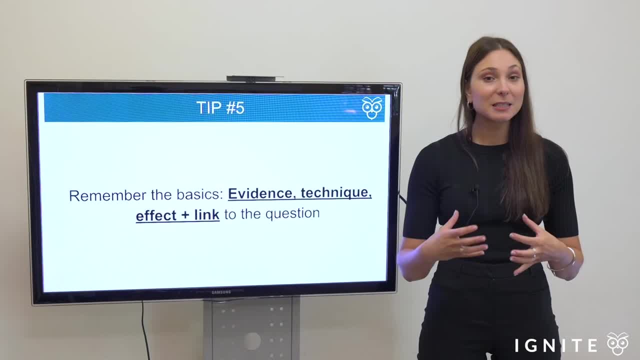 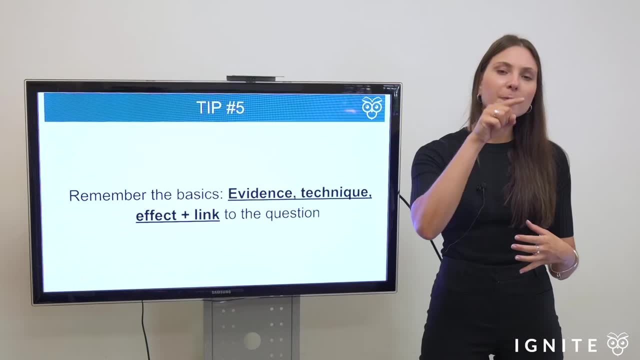 where the technique has been mentioned, Make sure you're actually showing that you can identify where in the text that technique is taking place. If you've picked quite a long quote, make sure you pinpoint within that quote where the technique actually is. The marker needs to. 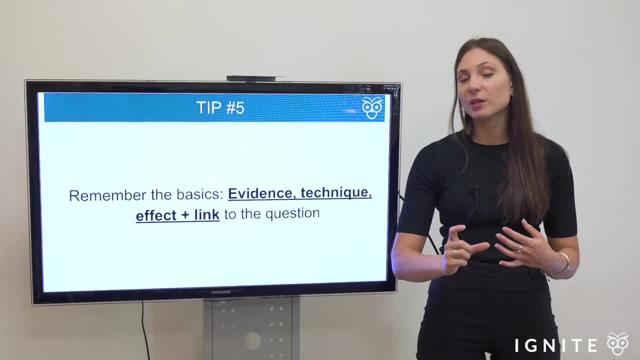 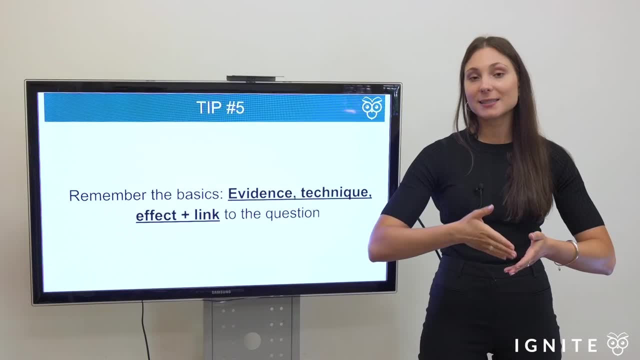 be satisfied that the student actually understands how analysis is working in the text and you're not actually circumventing the need to analyse specifically, show where the technique is taking place and explain the effect And, of course, most importantly, the effect that you're unpacking.